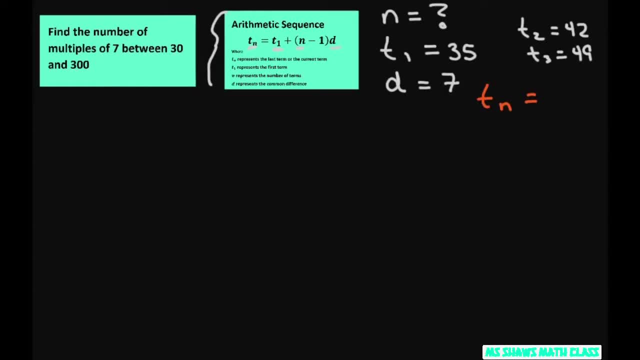 a little harder to find, And a good way to do that is first of all, just do long division and take 7 into 300.. Now if you do that, you're going to get 4 here. 4, that's 28. And we're. 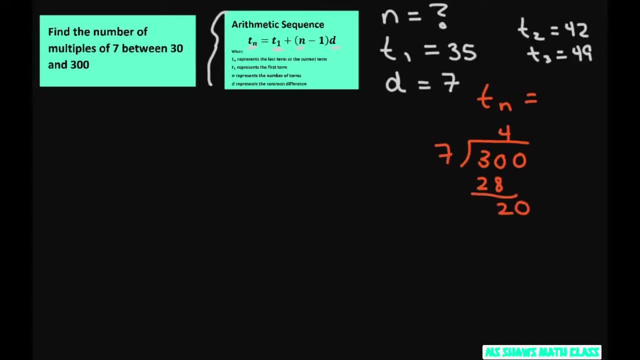 going to subtract, You get 20.. And then this will be 2. And that's 14.. Subtract: You get 6.. So the remainder is 6.. So what you can do is either take 300 minus 6,, which gives. 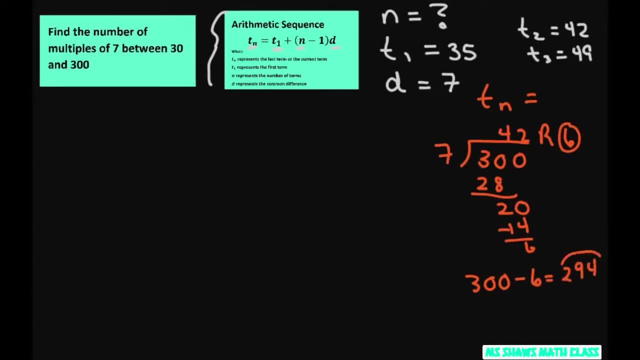 you 294.. That's going to be your last term, because you're subtracting the remainder, Or what you could do is just take 7.. 7 times 42. And that will give your last term. So 7 times 42 equals 794.. So our last. 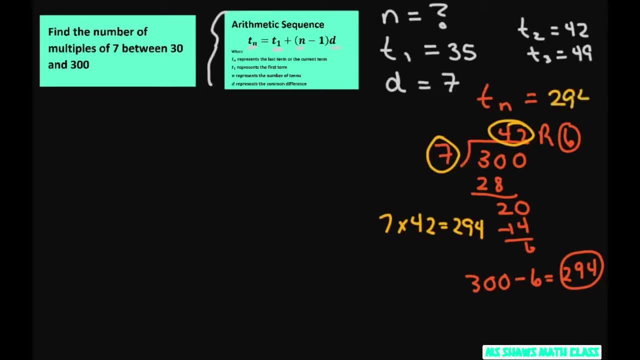 term is going to be 794.. And then you just use your formula, So we have 294 equals. our first term is 35 plus N, and this is the part we don't know. minus 1 times your common difference, or your multiple, is 7.. So, simplifying that, we're going to get um if you add 35. 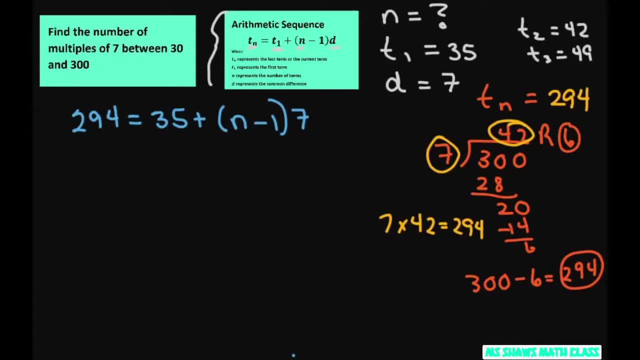 to both sides. Let's see, Let's just do it this way. So you get 294 equals 35, plus 7N minus 7.. Alright, So this is going to end up giving you 7N equals 266. so 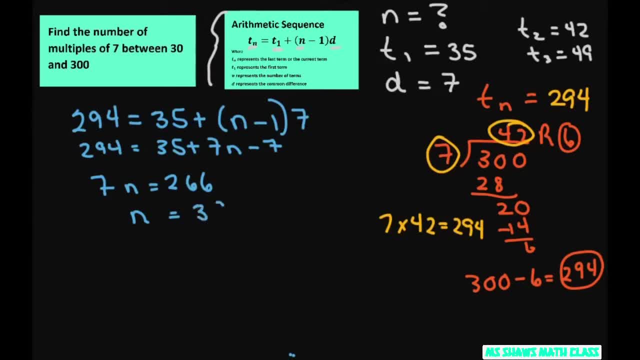 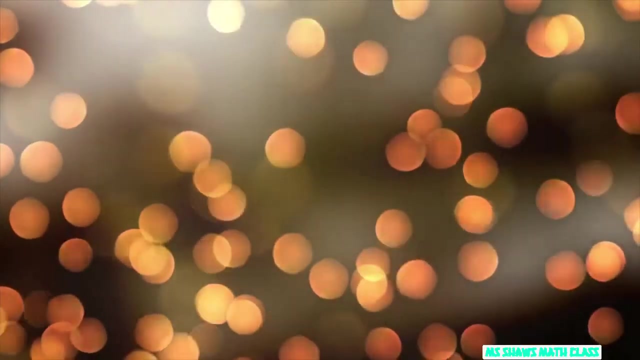 n equals 38 and that's your final answer. you can always plug it back in and check and check it back into the original and see if you get 294. that's it, thank you, have a nice day, bye, bye, the.